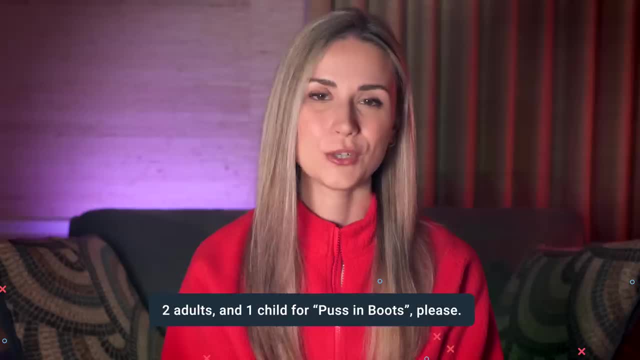 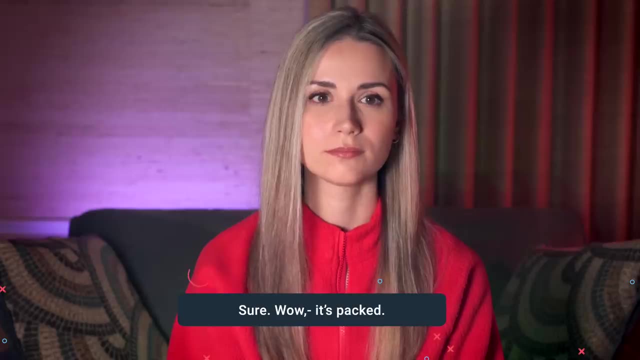 I'm not Okay. what would you like to watch tonight? Two adults and one child for Puss in Boots, please? Awesome. Could you choose your seats on the screen please? Sure, Wow, it's packed. Oh yeah, it usually gets pretty crowded in winter. 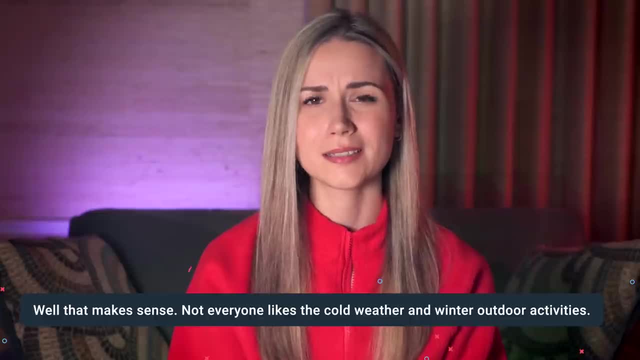 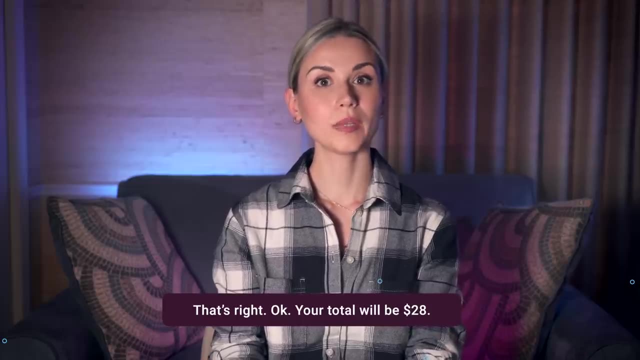 plus, it's a federal holiday. Well, that makes sense. Not everyone likes the cold weather and winter outdoor activities. That's right. Okay, your total will be $28.. All right, there you go, Thank you, It's theater number five, to your right. 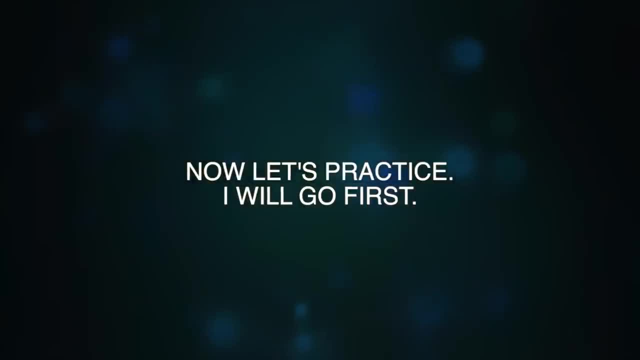 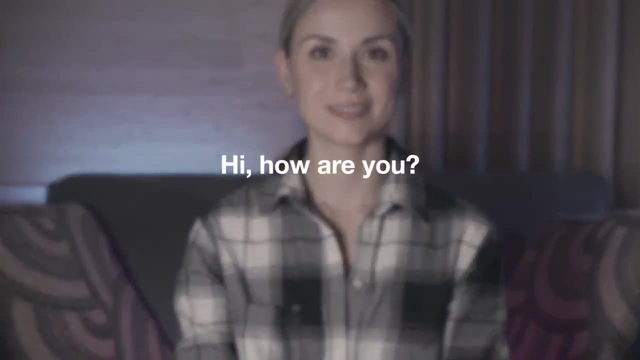 Enjoy the movie. Enjoy the movie. Thank you so much. Have a good one. Now let's practice. I will go first. Hi, how are you doing? Welcome to AMC. Are you paying cash or card? Are you a member? Okay, what would? 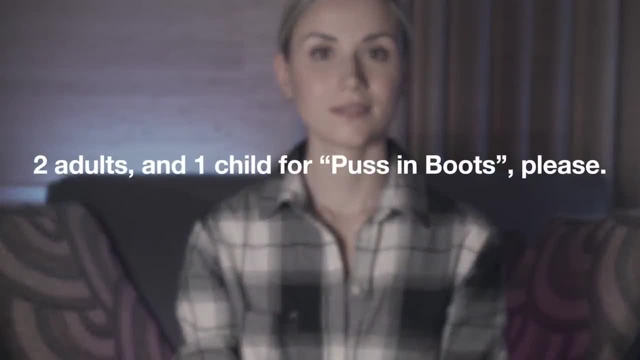 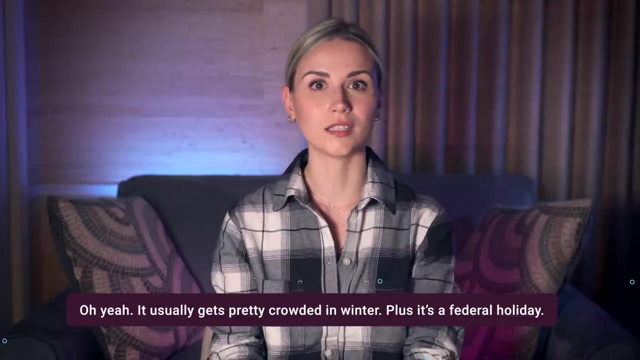 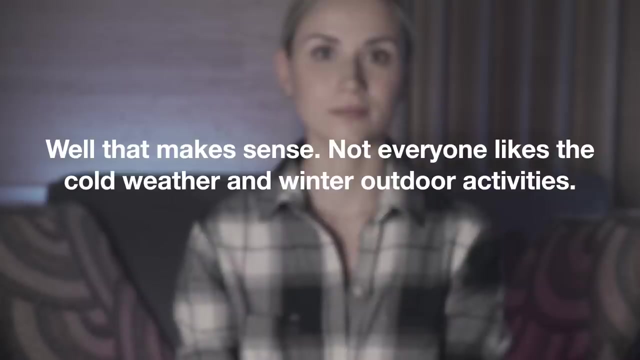 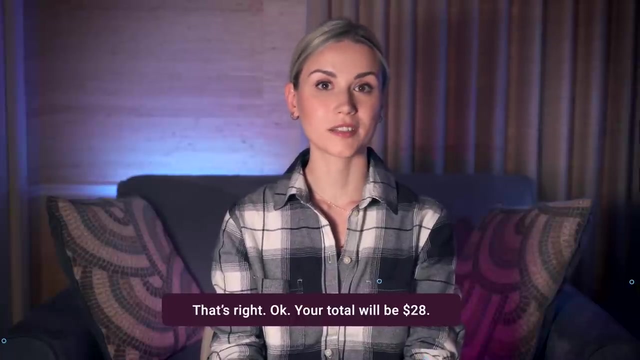 you like to watch tonight? Awesome. Could you choose your seats on the screen please? No, I'm not. Yeah, I'm not. I don't know how to use ID cards any Well, if you don't wanna crazy, I would appologize on this. If I might ask you: which theater do you like to watch? Get back in theности. 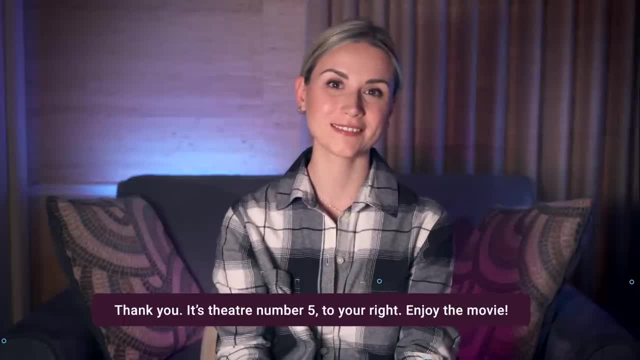 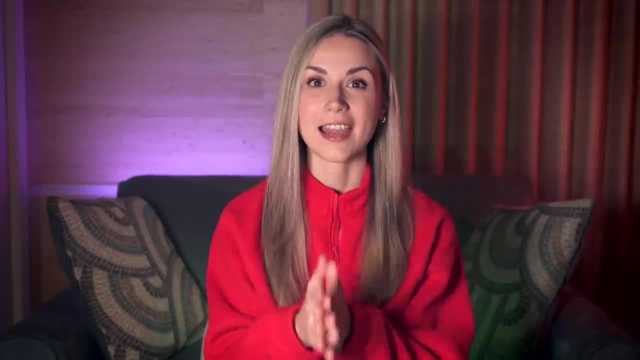 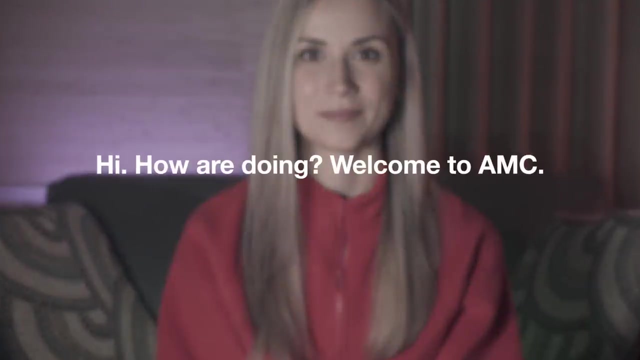 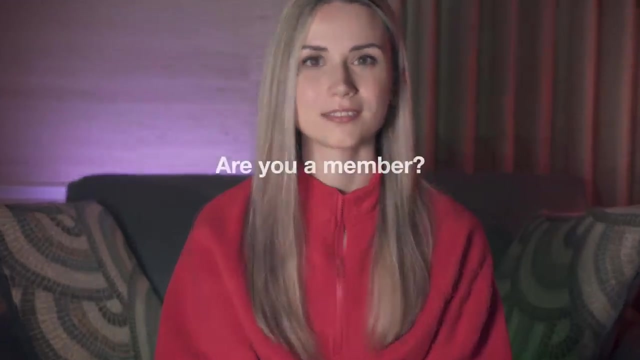 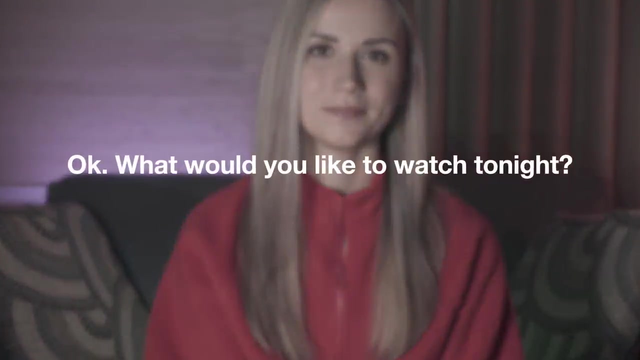 It's theater number five to your right. Enjoy the movie. Okay, amazing job everyone. Now we switch. You go first. Hi, how are you Card? No, I'm not Two adults and one child for Puss in Boots, please.